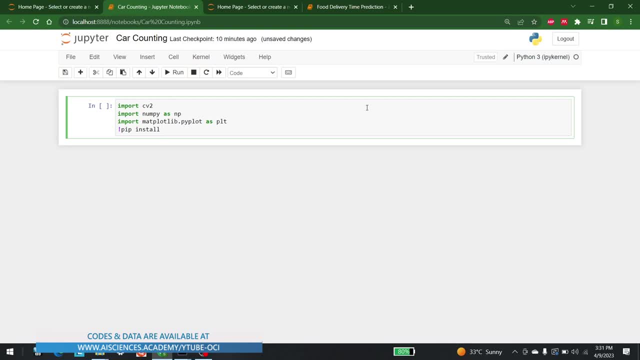 as well. you need to write pip, install CVlib. I already have that installed, So that's why I'll just import it. So let's import that. Import CVlib, and I already have CV2.. That's why I will import this one as CV. So let's run all of these, Okay. So now, after we are able to import, 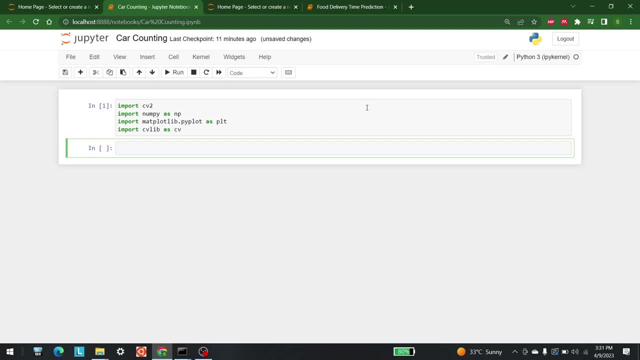 all of these libraries. as you can see, we are going to import the object detection, you know, bounding box, Right, And it is available in this library, Right? What do we want? We want to what you're going to tell us that this is the car, This is something Alright, So for that. 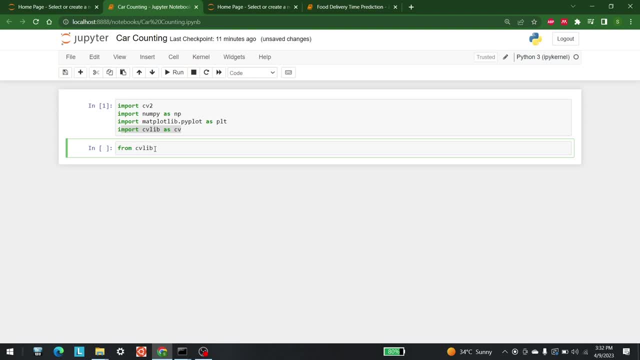 what I am going to do is I'm going to just write from CVlib dot: object: underscore detection: import, draw. underscore B-Box Right. So let's import that as well. And after that, what are we going to do is that we are going to import the code And we'll want to cat acquire 손ang when, let's say, they get a bit hard at these things because they're trying to go somewhere. haven't done what we want, So what does it do it instead of getting to bring in this, you know, which is distributedhof in the description over unstable? 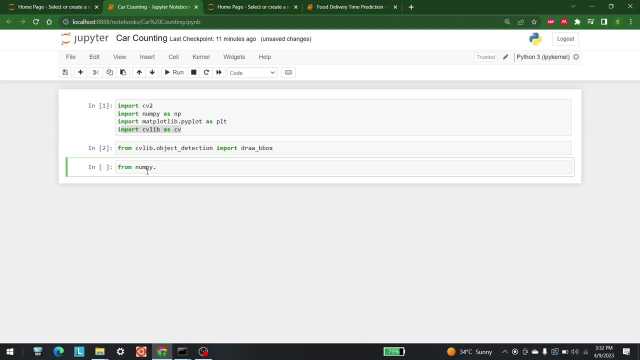 So it will walk out the vulnerable contract from that lib, from therition, Right, But we are going to numpy poly from numpy, which will be a polynomial, just right. so numpy dot, lib, dot, polynomial- sorry, polynomial- and i am going to import poly from here, okay, so, after doing that, it is now time. 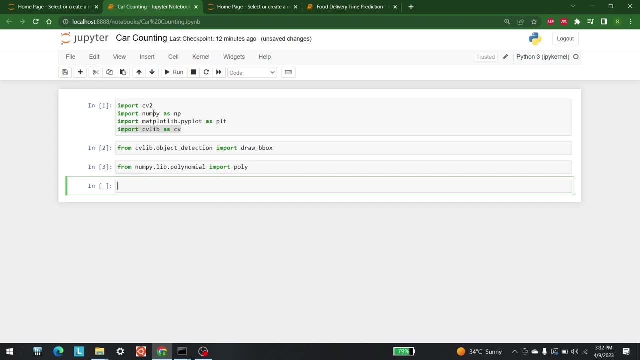 to import the image. so if you know about open cv, we can just use the cv2 dot im read command to import the image, right? so image is equal to cv2 dot im read and here i am going to give the name that as cars dot jpg. okay, so after doing that, what is the next step? 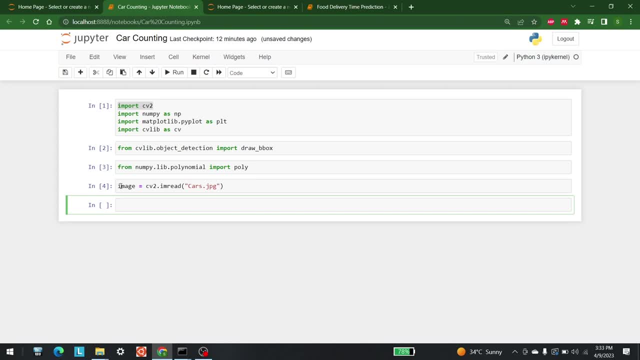 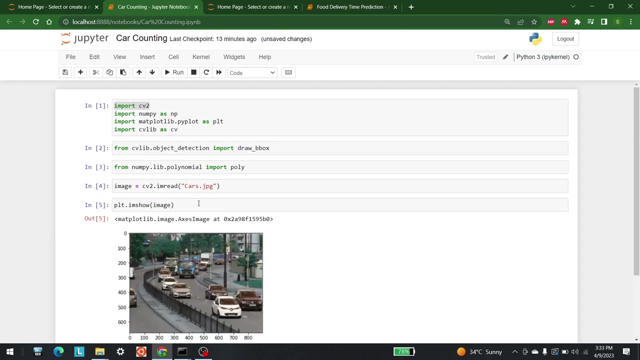 the next step is to, you know, make the bounding box around that image, right? so, uh, let's do that. we are going to write, uh, actually, let's first show you the- uh, you know image. so here i am going to write image and this is the image, right? 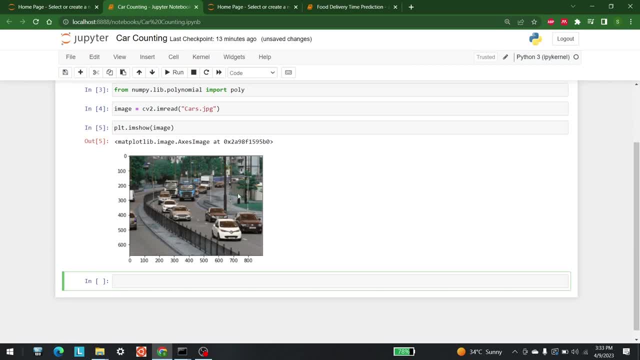 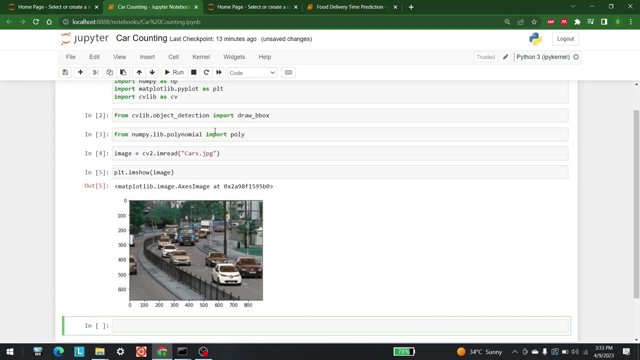 so these are all the cards that are available in this image. so we want bounding boxes around all of these cars. so what are we going to do? we are going to, you know, use the common object detector that is available in cv, right. what is cv? cv is the cv lib right? so we are going to detect. 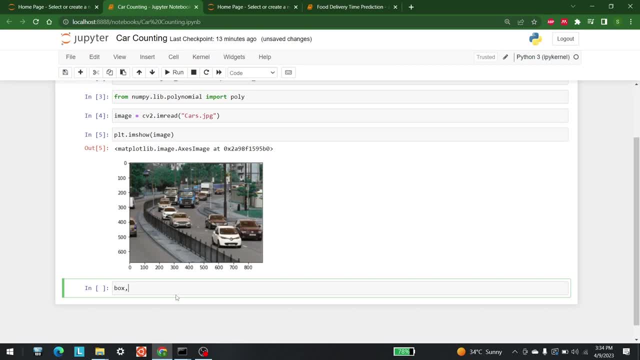 through that. so let's do that box comma label. it is, you know, available open source, so we do not have to make anything right. so cv dot detect underscore, common underscore objects. and here i am going to write image. after that i am going to write: output is equal to draw. 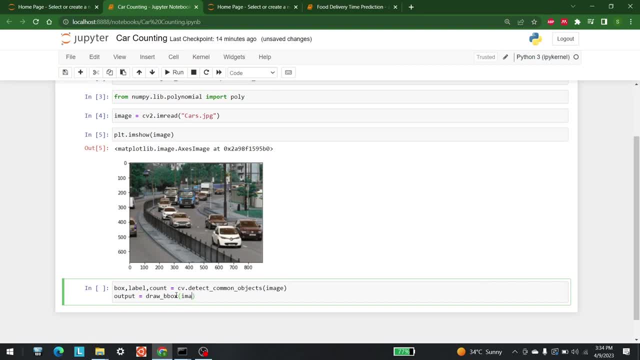 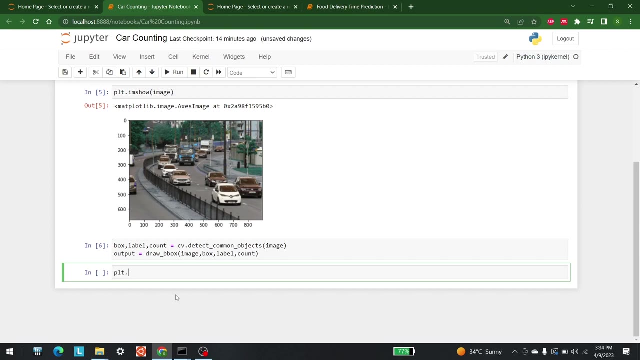 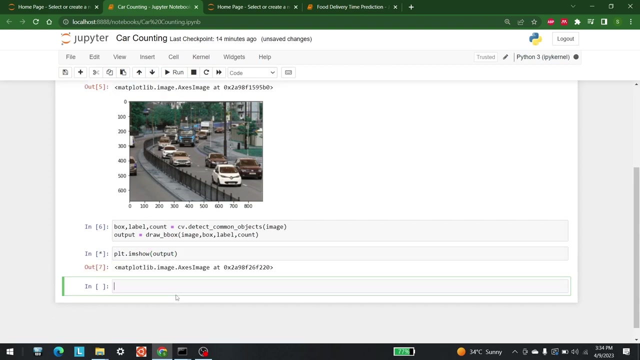 underscore b box, and here i am going to write image, comma, box, comma, label, comma, count, right, so let's see what we get. so now i am going to show you the output as plt, dot. i am show and here i'll give you the output. and there we go. as you can see, we have these bounding boxes. 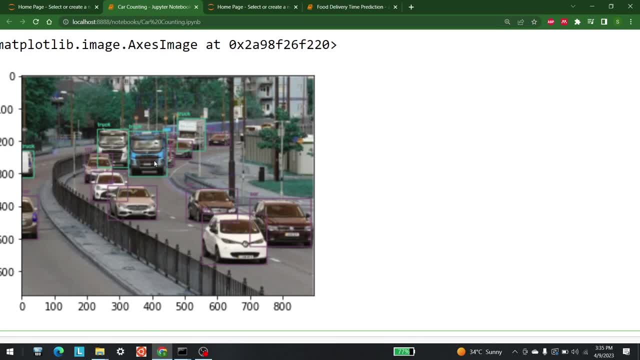 outside of each car. maybe we are not able to see it completely right, so now, as you can see, it is saying that this is a card, this is a car, this is a car. here, due to the display system, we are not able to completely see that car is written here, but it is right and it is writing: this is a 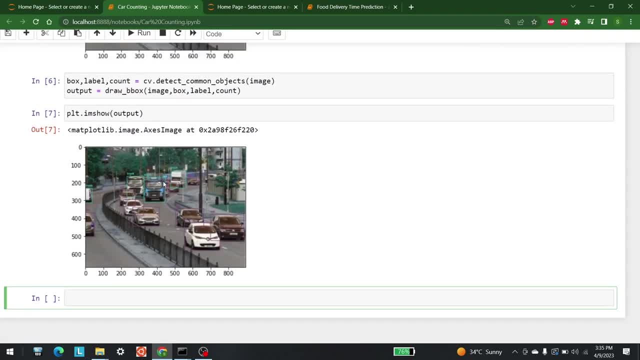 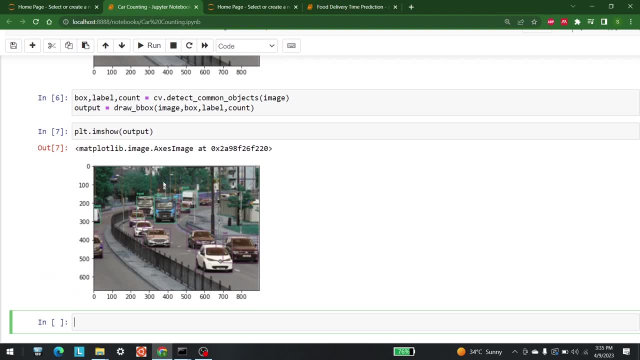 truck. this is a truck, this is a truck. so there we go. this is the way to detect, you know, cars in any image, right? so, as you can see, it was a very easy code as well, right? of course, we can also see the count of the number of cars in this, right? so, for that, what i am going to do is i am going to